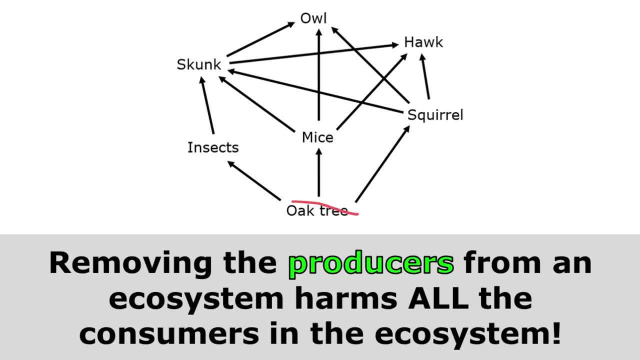 The food sources. areсы mogę 할게요. combines encourages the consumers to be in an ecosystem. However, after drying of all of these entitled to their food and promoting resources, issues have been恐惗one. So if I cut down all the oak trees in this ecosystem, that means there's no food or 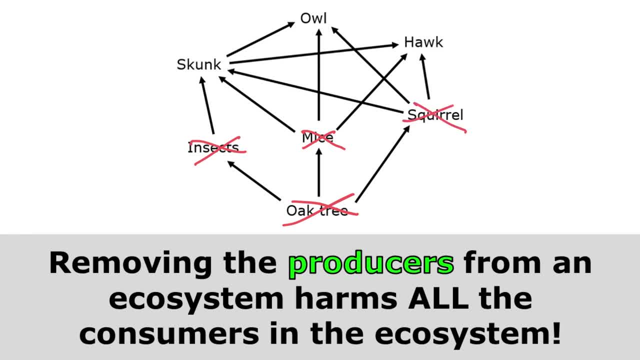 shelter for insects, dinosaurs, mice or squirrels. So all of the insects, mice and squirrels that use the oak tree as a food source are going to have to leave or they'll die. But because all of the insects, mice, 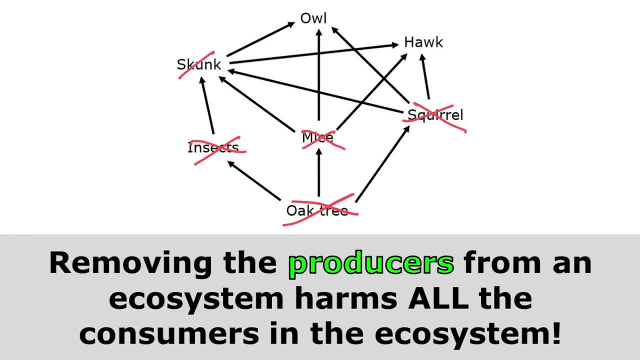 and squirrels are gone. that means that there's no longer any food for skunks, owls and hawks. So you can see that by taking away the producers, I've caused a domino effect that causes all of the consumers to either have to leave to find food elsewhere or die. 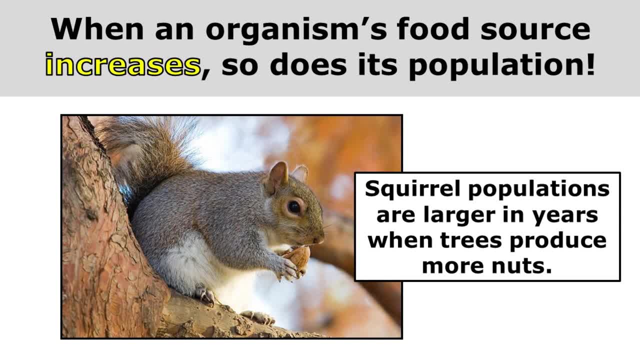 So we've been talking about what happens when we take away an organism's food source, But it's also true that when an organism's food source increases, so does its population. Squirrel populations are larger in years. when trees produce more nuts. That's because they have more food, and so more squirrels can survive because there's more food for all of them to eat. 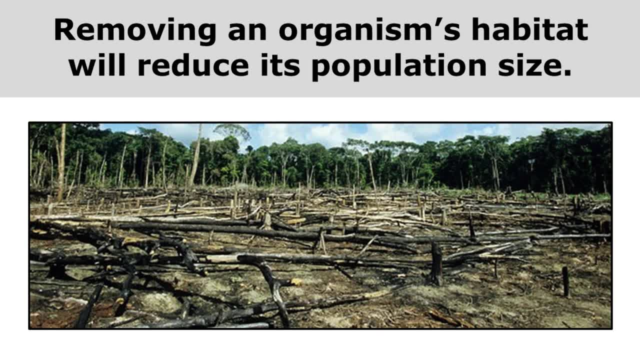 So another way that humans can actually harm organisms is by taking away their habitat. So removing an organism's habitat will reduce its population size, And here you see that these trees have been chopped down and deforestation is a huge problem that really harms these forest ecosystems. 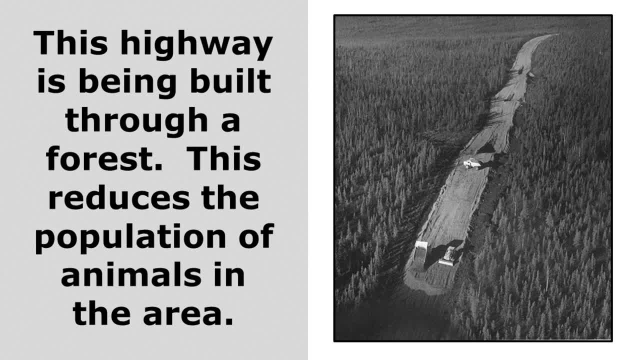 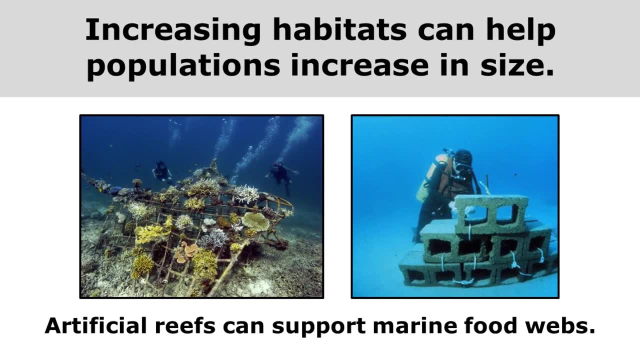 And here you can see a highway being built, and this highway is being built through a forest And this reduces the population of animals in the area, because their habitat and their food source for many of them are being taken away. But increasing habitats can help populations increase in size. 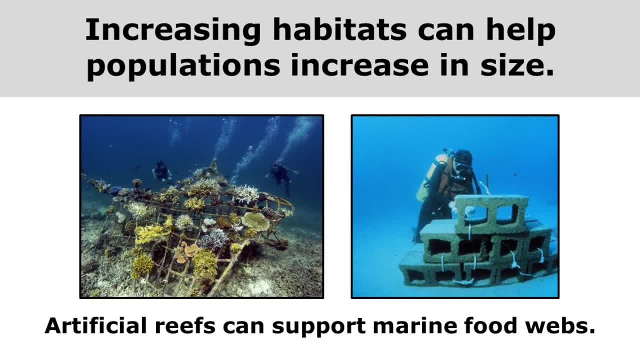 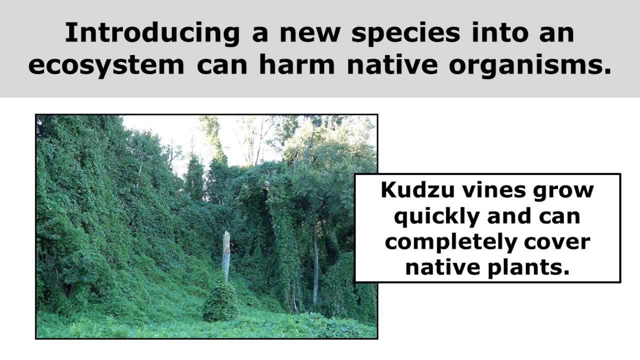 And here you see two examples of man-made artificial reefs, And artificial reefs can support marine food webs And this helps INCREASE the populations of marine organisms. Introducing a new species into an ecosystem can harm native organisms. Kudzu vines were introduced into this ecosystem and kudzu vines grow quickly and can completely cover native plants. 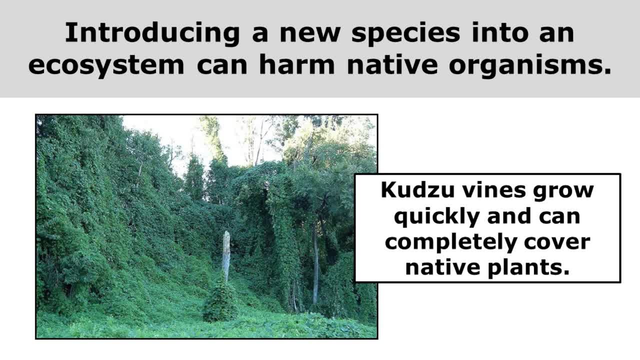 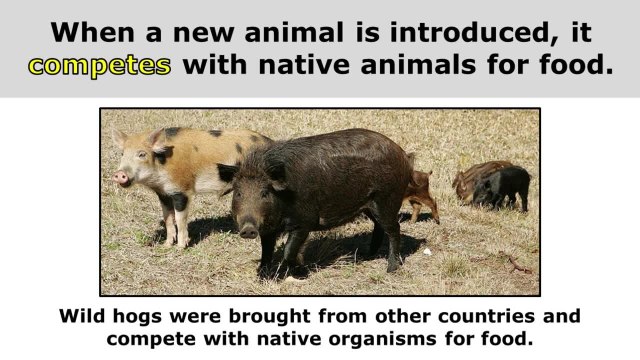 And that KILLS the native plants that they cover and reduces the population of plants in this ecosystem. When a new animal is introduced, it COMPETES with native animals in the ecosystem. When a new animal is introduced, it COMPETES with native animals in the ecosystem. 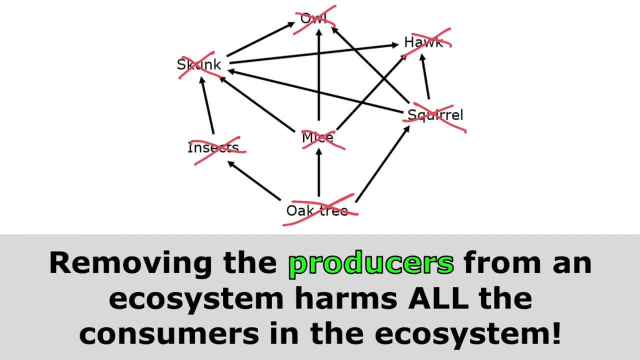 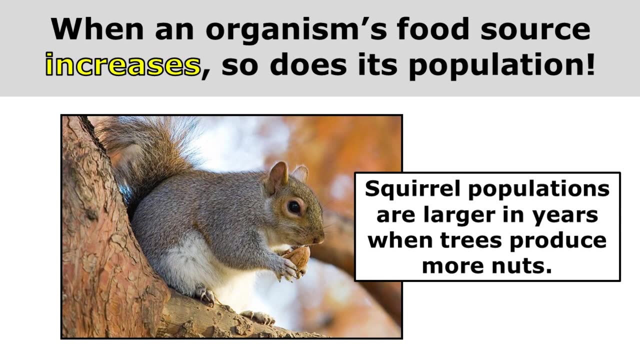 What happens if you cut down a population. So you can see that by taking away the producers, I've caused a domino effect that causes all of the consumers to either have to leave to find food elsewhere or die. So we've been talking about what happens when we take away an organism's food source. 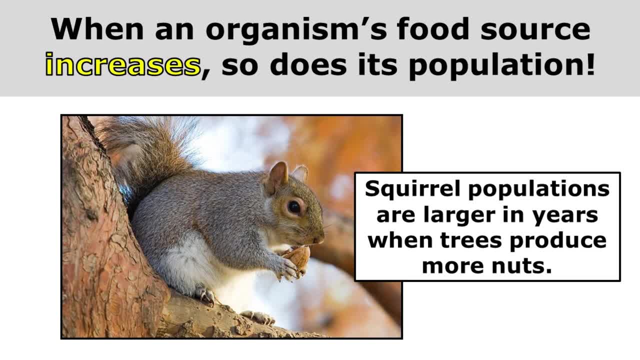 But it's also true that when an organism's food source increases, so does its population. Squirrel populations are larger in years. when trees produce more nuts, That's because they have more food, and so more squirrels can survive, because there's more food for all of them to eat. 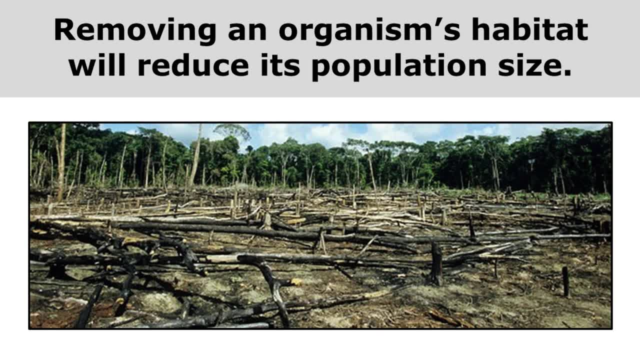 So another way that humans can actually harm organisms is by taking away their habitat. So removing an organism's habitat will reduce its population size, And here you see that these trees have been chopped down and deforestation is a huge problem that really harms these forest ecosystems. 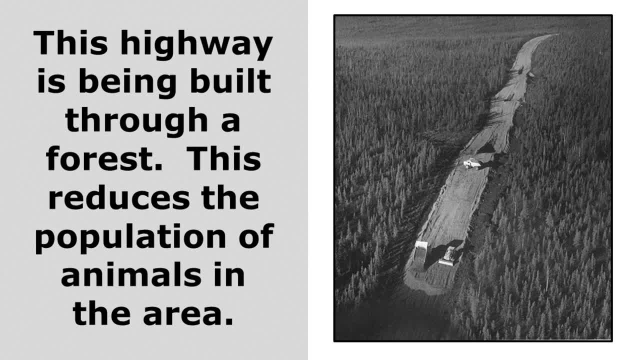 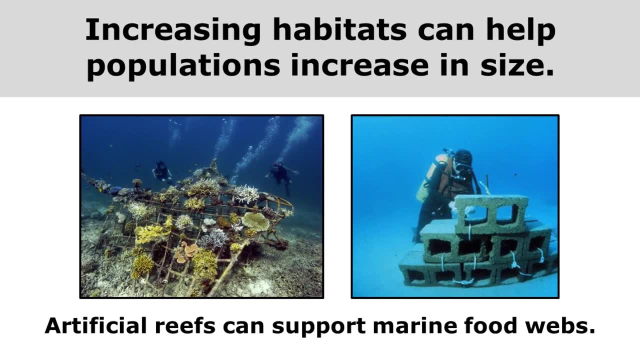 And here you can see a highway being built, and this highway is being built through a forest And this reduces the population of animals in the area, because their habitat and their food source for many of them are being taken away. But increasing habitats can help populations increase in size. 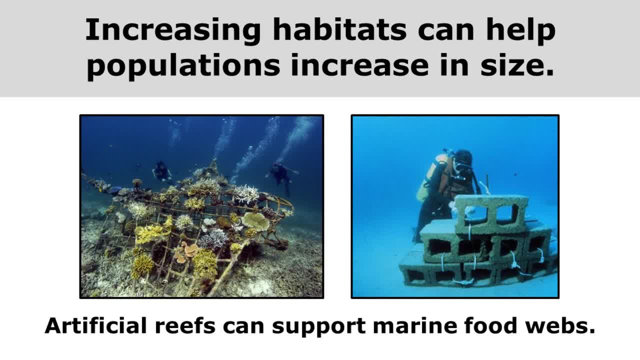 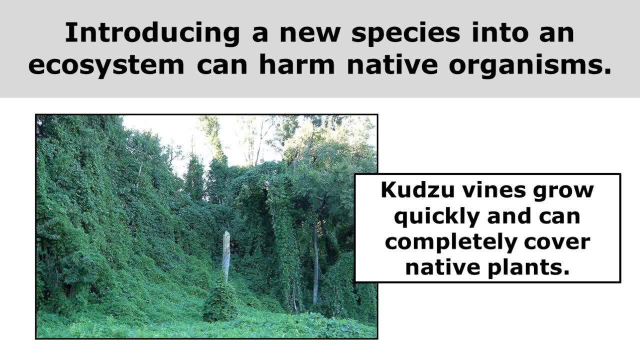 And here you see two examples of man-made artificial reefs, And artificial reefs can support marine food webs And this helps INCREASE the populations of marine organisms. Introducing a new species into an ecosystem can harm native organisms. Kudzu vines were introduced into this ecosystem and kudzu vines grow quickly and can completely cover native plants. 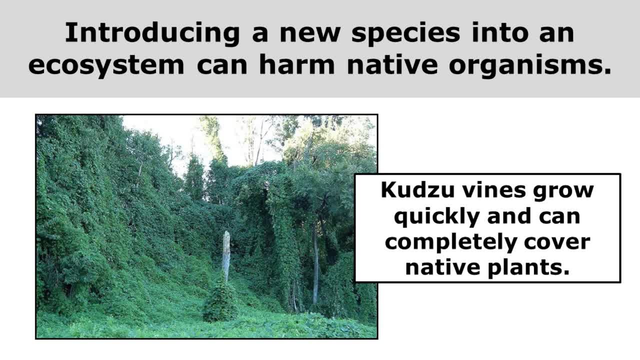 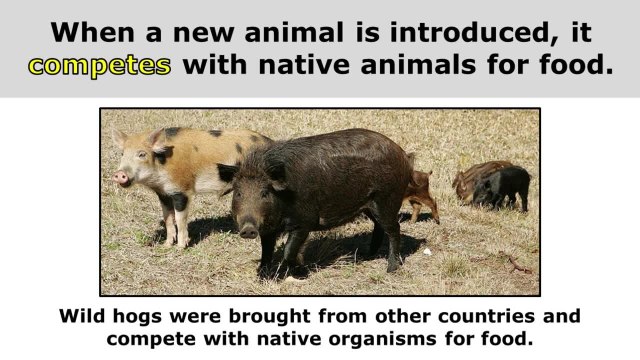 And that KILLS the native plants that they cover and reduces the population of plants in this ecosystem. When a new animal is introduced, it COMPETES with native animals in the ecosystem. When a new animal is introduced, it COMPETES with native animals in the ecosystem. 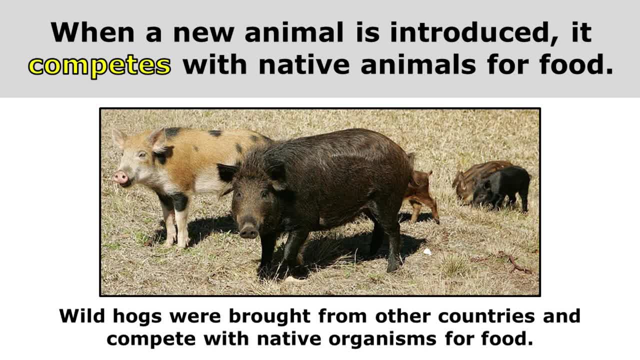 Sand Ice Tutaj is sometimes referred to as 순رес, which means the r? Lilater of wilderness. Wild Hogs are a big problem in Texas. Wild Hogs were brought from other countries and compete with native organisms for food. When animals feed on grasses and other plants, we call it GRAZING. 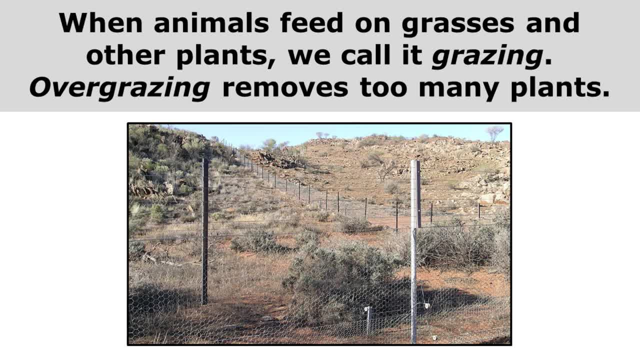 OVER Grazing removes too many plants and in this picture you can actually see the effects of overgrazing. And in this picture you can actually see the effects of overgrazing. So animals on this side of the fence have been allowed to eat too many of the plants.